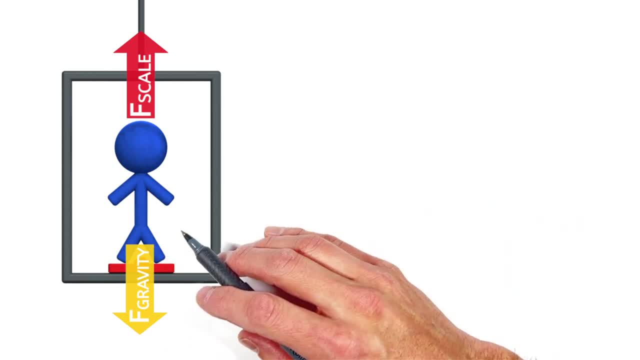 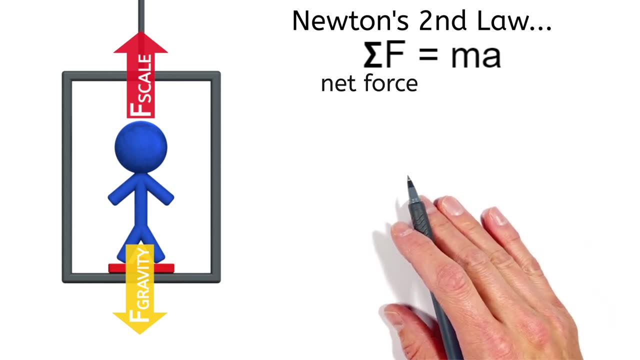 behind a free body diagram like this is that it helps us apply Newton's second law to the problem. See, the second law is an equation that says the net force or sum of all forces acting on an object is equal to that object's mass times acceleration, And a free body diagram is really. 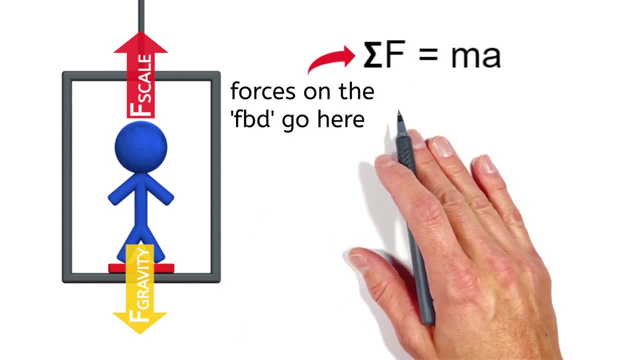 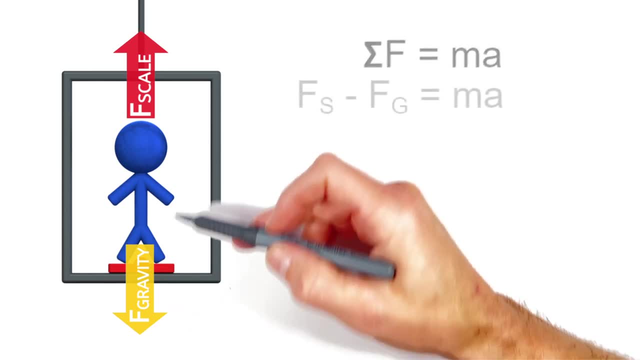 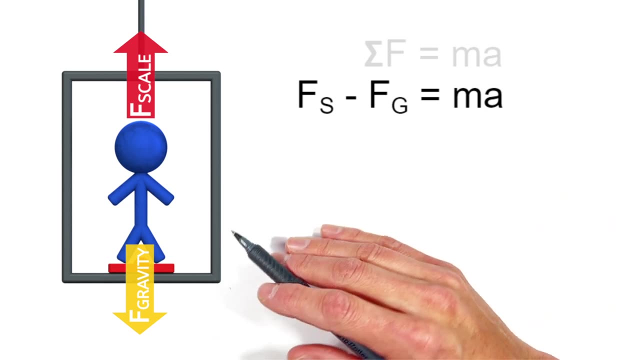 just a picture of the left half of Newton's second law, or what we'd call the net force. So to solve for the reading on this scale, we're going to set the sum of these two forces equal to the person's mass times. acceleration. Now, force is a vector, meaning direction matters. So we have 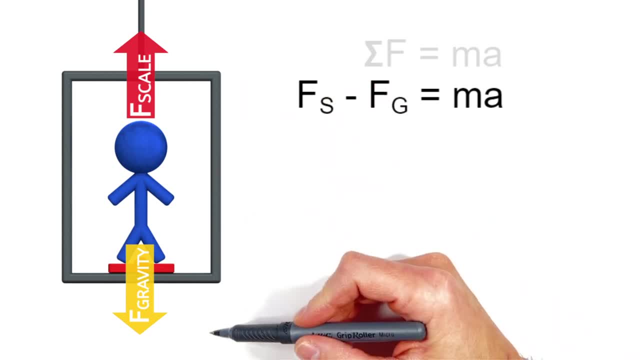 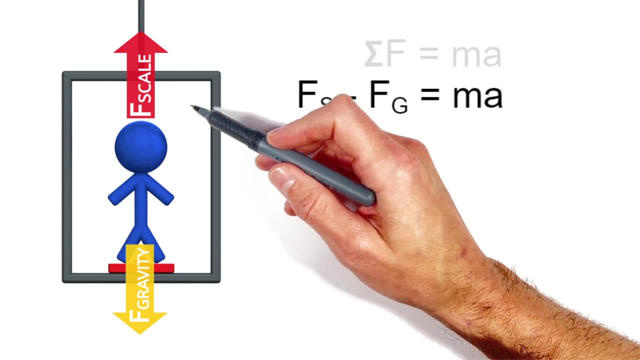 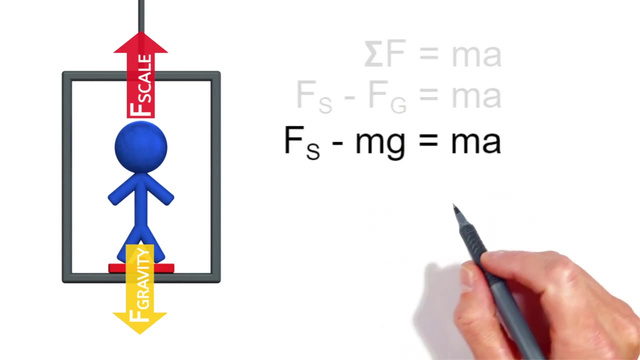 to make a distinction between forces up and forces down. So if we say up is the positive direction, this upward force by this scale is positive and the downward force by gravity is going to be negative. And rearranging this, this leaves us with an equation that relates the reading on this scale to the acceleration of the. 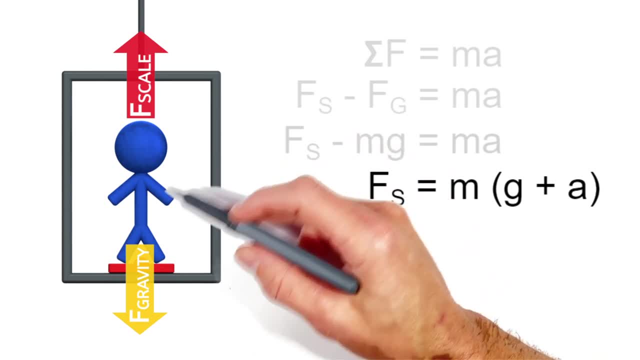 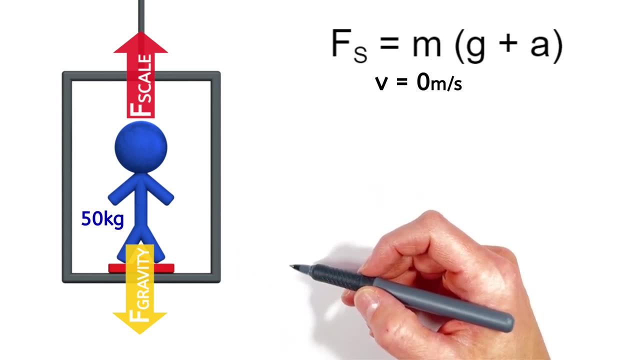 person in the elevator. So let's look at a simple scenario where this elevator is at rest and our person- let's give them a mass of 50 kilograms- is just standing there. In this case, the acceleration of the elevator is zero. So, going back to our equation, plugging in the 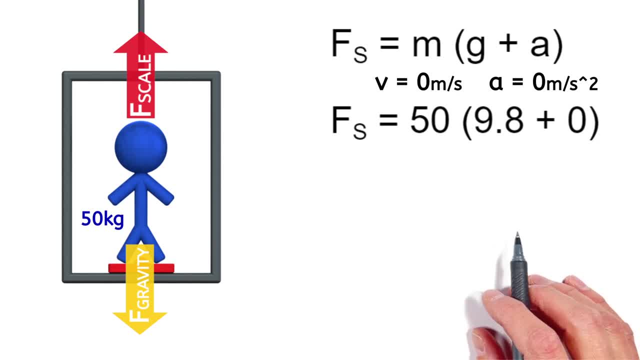 m, the mass is 50 kilograms g, the acceleration due to gravity is 9.8, and a is equal to zero in our equation. we find this scale is going to read a value equal to the weight of the person, or 490 newtons, And there's no big surprises here. You might expect a scale to read the weight of. 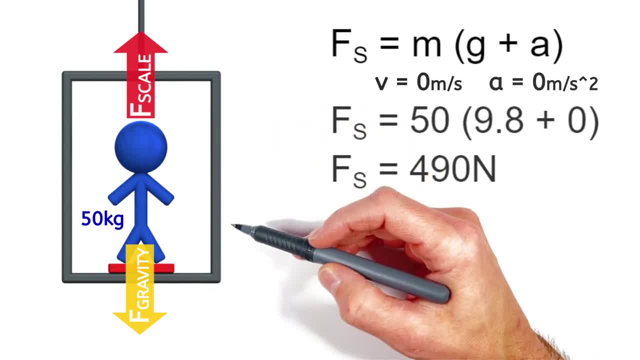 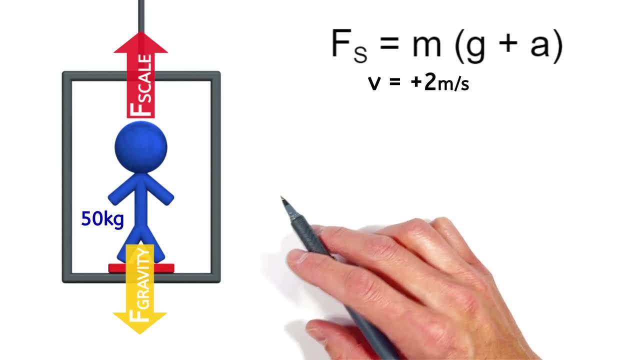 whatever you put on it. But next let's say this elevator is moving steadily upward at two meters per second. Now you may be in the middle of a elevator and you're going to be able to read the that there now has to be more force upward on the person because they're moving up. But remember, 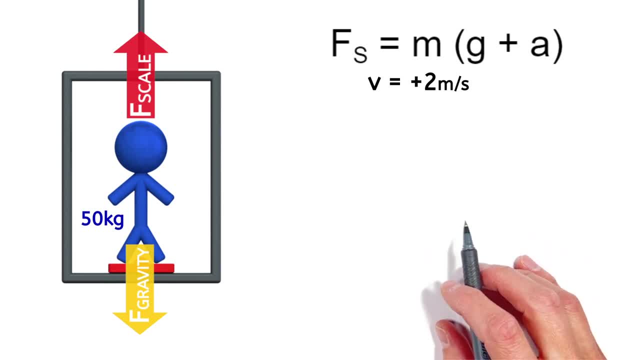 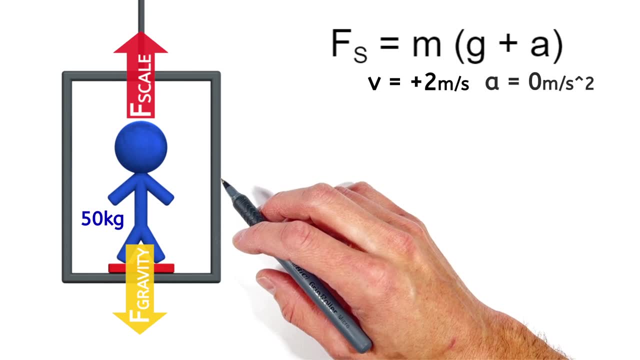 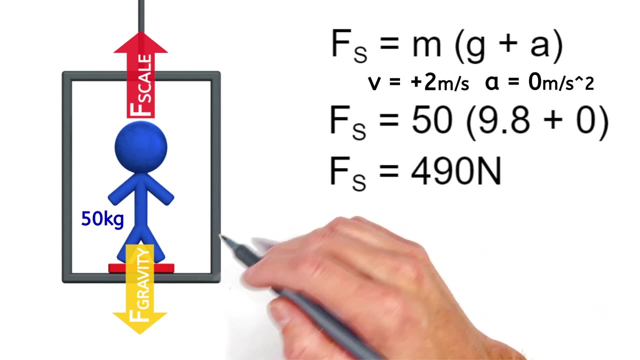 going back to our equation, the force on the person is dependent on their acceleration, not on their speed. A over here is still zero meaning. none of this math changes The person in the elevator. they feel completely normal. So let's change the motion of this. 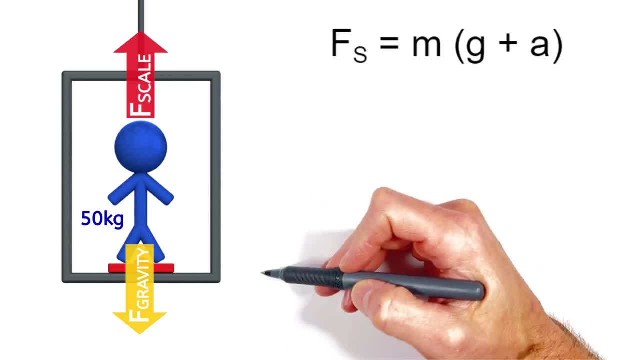 elevator again, And this time let's make this elevator accelerate upward at three meters per second squared, And this is where things start to get a little weird. So in order to make the person accelerate upward, there has to be more force up on the person than down Or going back. 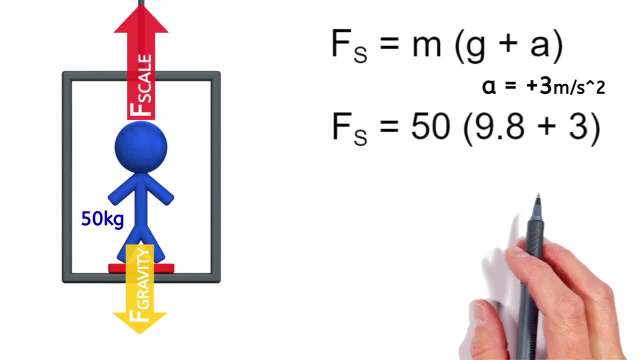 to our equation. if you plug in a is positive three and say it's positive because it's upward, the force on the scale will be 640 newtons, And it's not that the person actually weighs more. Remember weight's always mg. So for this, 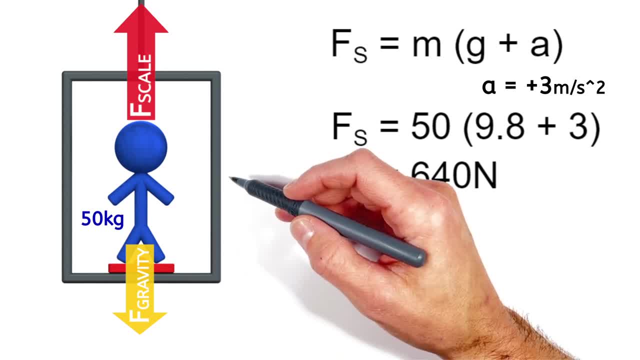 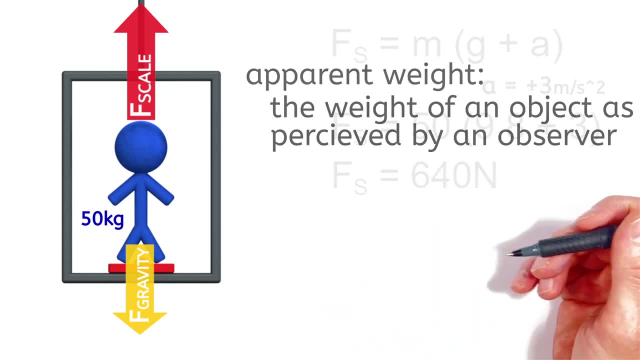 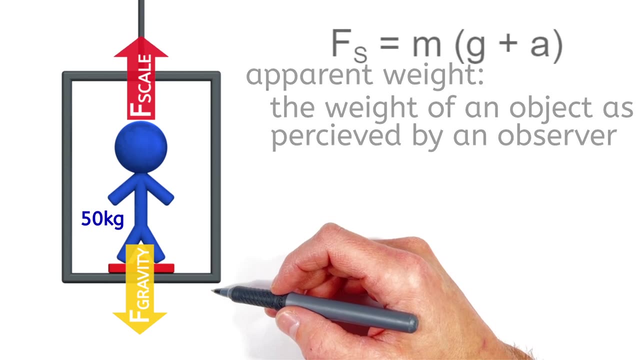 that's 490 newtons, but our scale reads more. and what's critical is, the person will actually feel heavier, and that feeling of weight is what we call their apparent weight. now, if we change this and have the elevator accelerate downward at 3 meters per second, squared going back to our 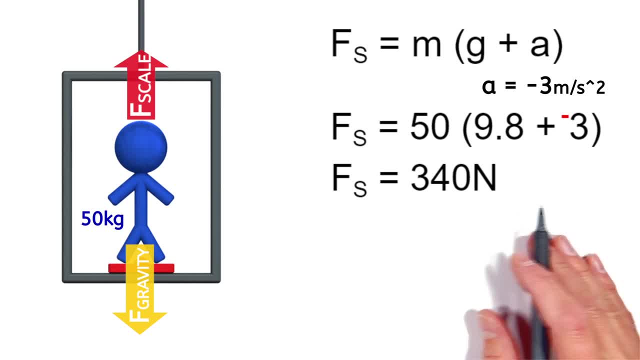 equation a is now equal to negative 3 because it's accelerating downward or in the negative direction, and the reading on the scale, or the apparent weight of the person, is 340 newtons. our person over here feels lighter, even though gravity is unchanged. it's still mg or 490 newtons. now, the idea that you can't 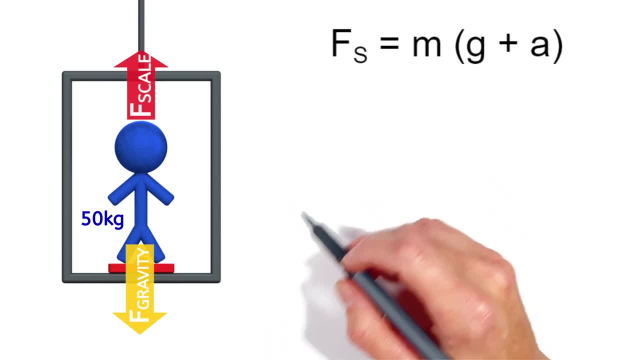 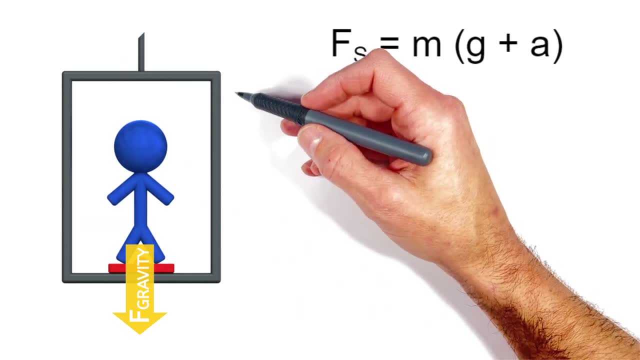 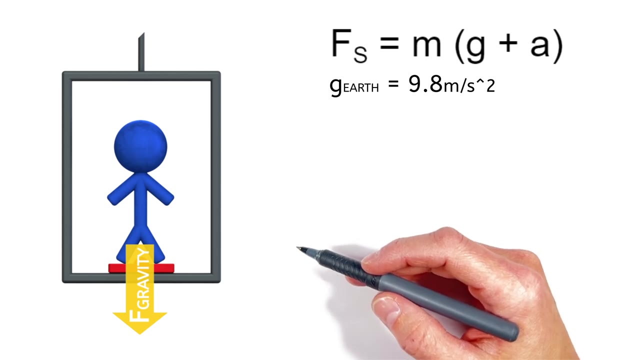 feel gravity and instead you feel your apparent weight can be hard to wrap your head around. so let's take this scenario one step further. let's cut the cable of this elevator so that the elevator free falls downward. any object and free fall on the surface of the earth accelerates downward at roughly 9.8 meters per 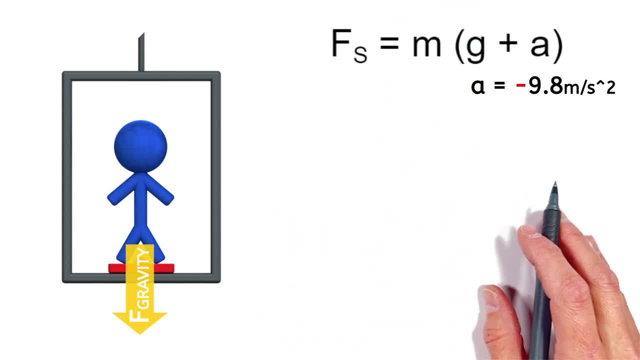 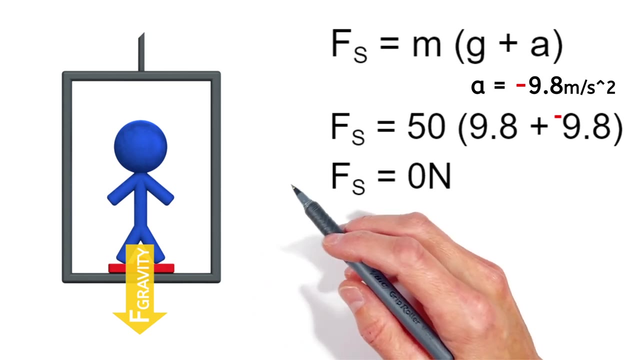 second squared, so plugging negative 9.8 into our equation for a, we find the force by the scale on the person must equals zero, meaning nothing is holding this person up there and free fall just like the elevator. but the important thing here is what this person feels. imagine this person just woke up from a nap with no. 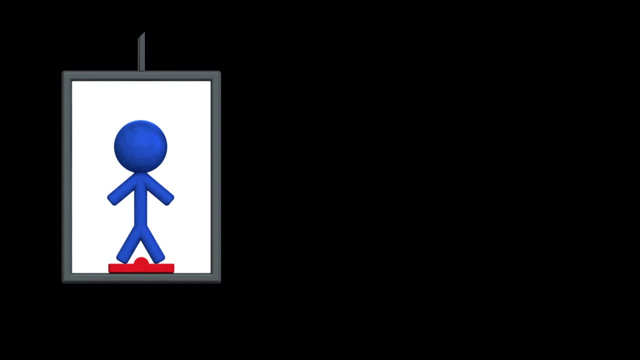 idea they were in a free-falling elevator with no knowledge of the elevators motion and nothing holding them up. the person would just float around and fall down the elevator with no knowledge of the elevators motion and nothing holding them up. the person would just float around.